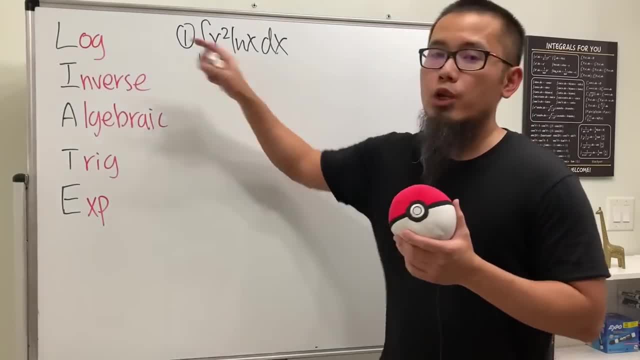 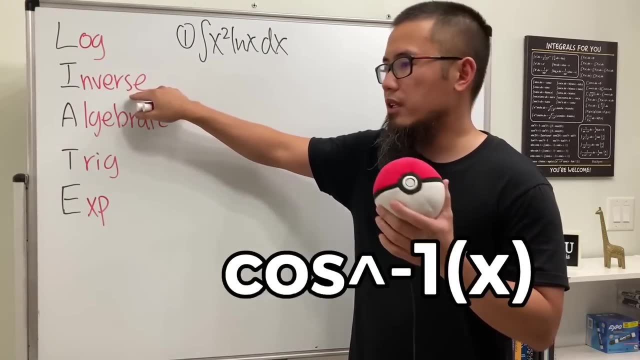 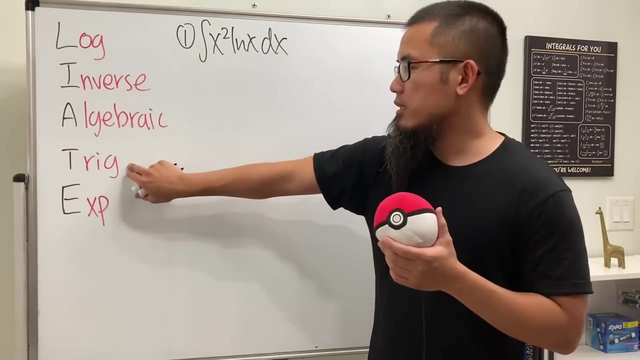 in this order. If you see log functions in your integral, you choose this to be differentiated. Next is the inverse functions, such as inverse tangent, inverse cosine, etc. And then next is algebraic, such as x to some power, and then next is sine cosine. 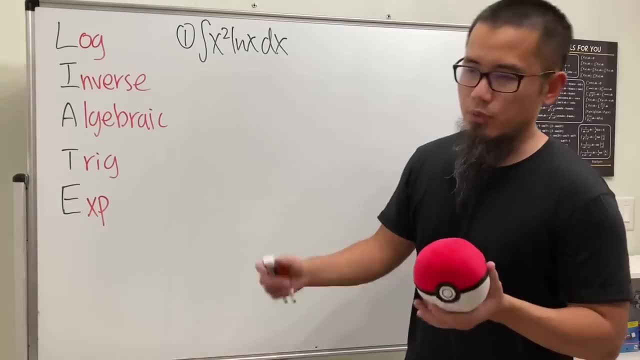 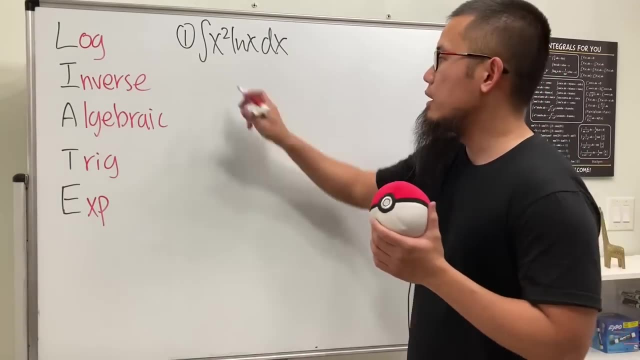 For the trig functions and lastly, we have the exponential functions, of course, e to the x and things like that, And, as we can see, we see log right away- so we'll choose that to be differentiated. So let's go ahead and put down a, d and an i plus minus to get ready. We will choose that. 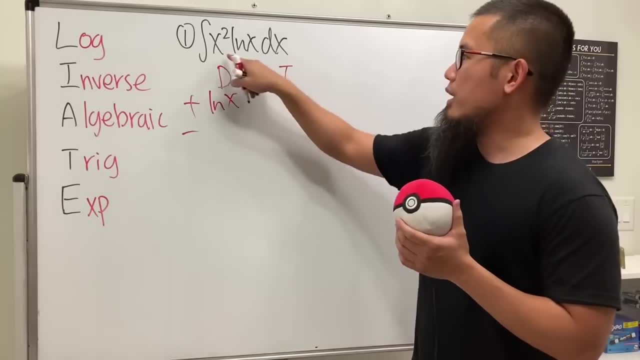 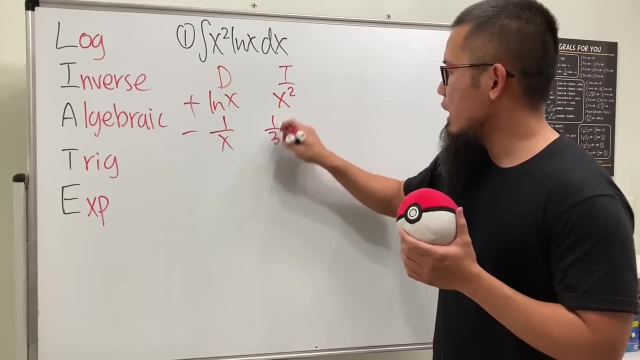 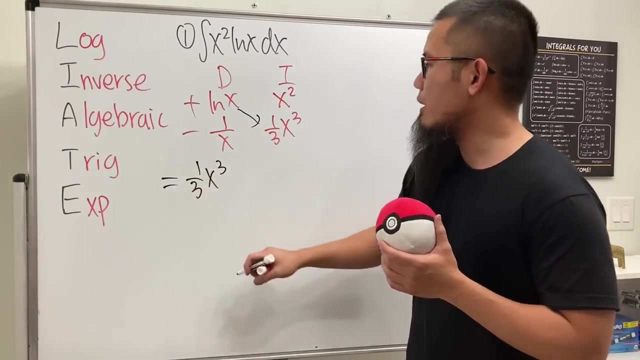 and there's no thanks to that. it's pretty easy. And of course we do x squared to be integrated. Go ahead, do that, Go ahead and do this. It seems pretty nice, and then let's just finish this and we will talk. So we get one third x to the third power times, ln x, and then we are going. 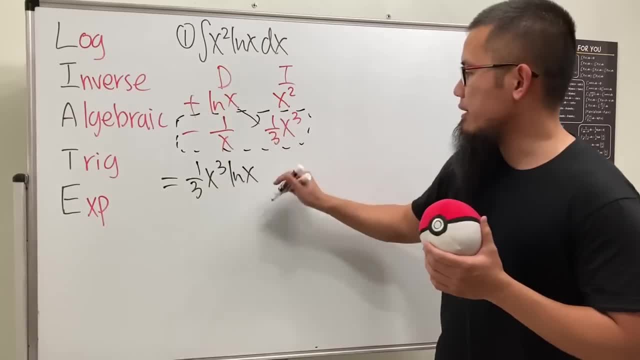 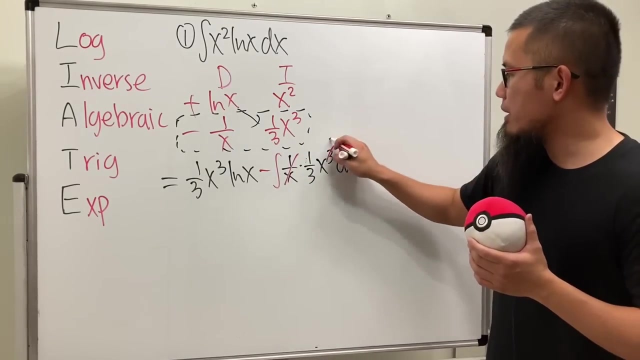 to multiply by these two things together and put that inside of an integral and subtract that Here we have 1 over x times 1 over 3, and then we have the x to the third power and let's put down the x, Cancel this out, and this right here becomes a 2 right. And of course, to integrate this we'll 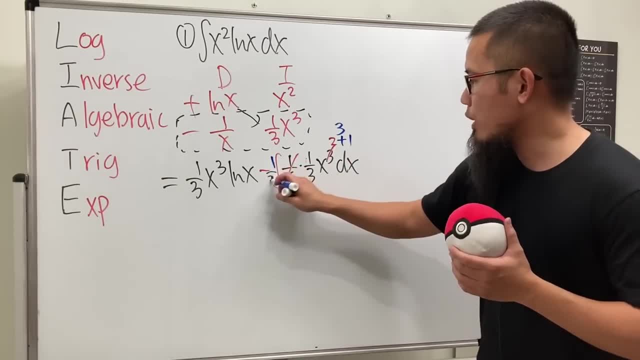 just add 1 to the power, which is 3 divided by the next power. So we have 1 over x times 1 over 3.. So we have 1 over 3.. So all in all this right here is just 1 over 3. x to the third power, ln x. 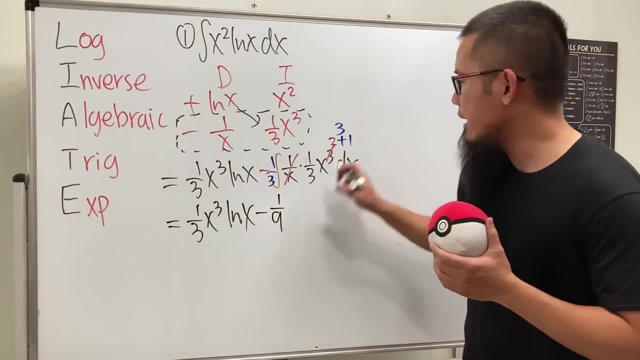 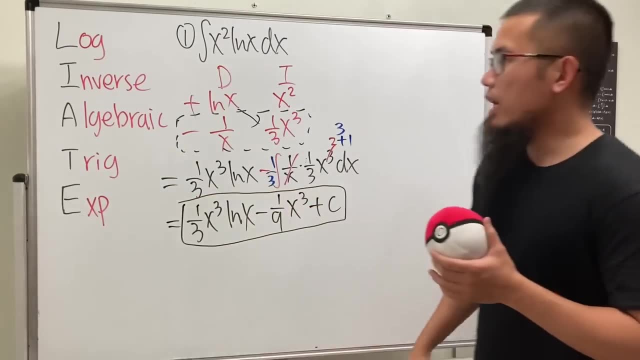 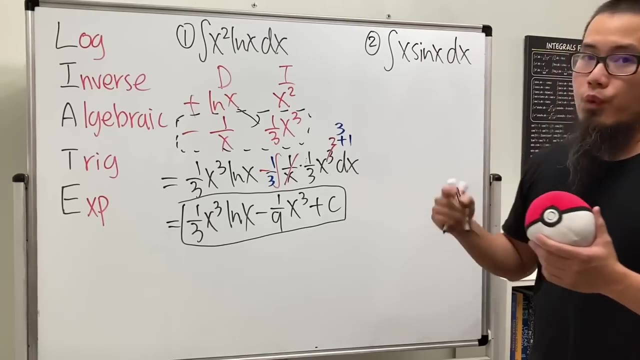 minus 1 third times 1 third, So 1 over 9 and then x to the third power Done. So this right here is very nice. And I can also give you guys another example. So if you are looking at the integral of x times sine x instead, Well, we don't have the log anymore. 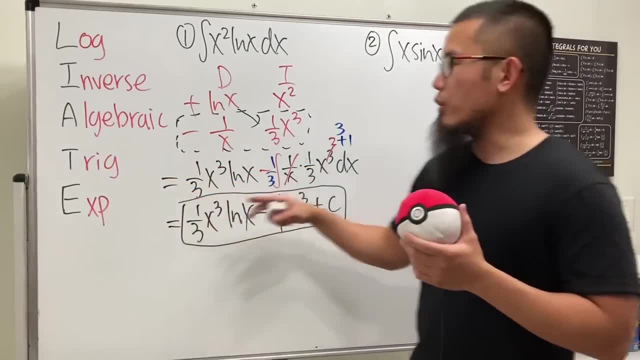 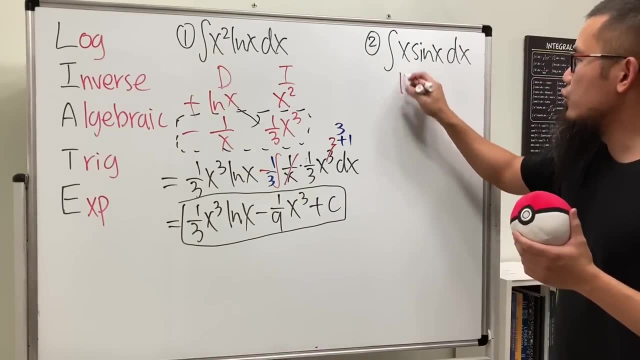 We have trig function, but you see it's down here. So that means we should actually choose x to the first power because it's above the trig function. So we'll choose the x to be differentiated. So let's just go ahead and put that down. 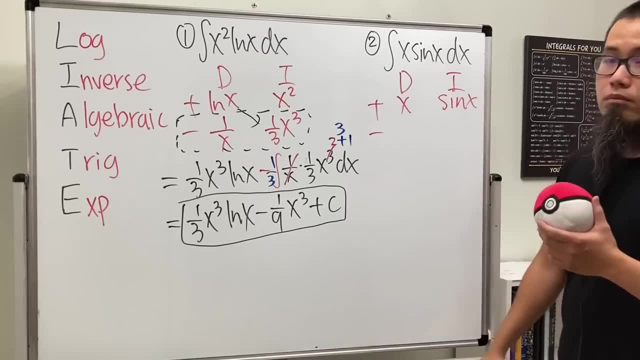 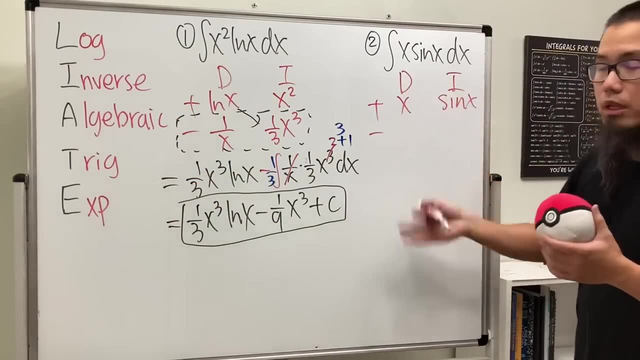 Put down the x right here and put down the sine x right here. Okay, x is algebraic, x to some power and trig is down below. So do this. And of course, you all know the integration by parts with the DI method, The DI setup. Do it once and then do it right here. 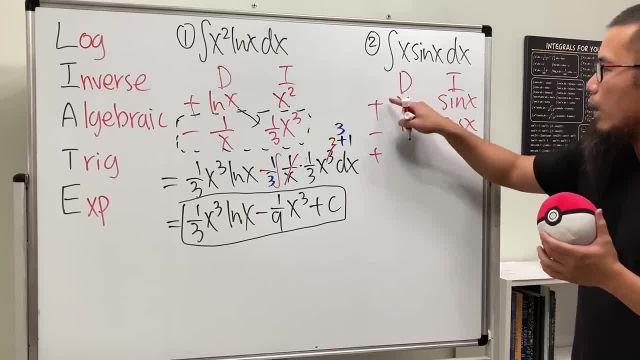 But we can get to zero, So that's fine. So let's do it again, So we have 1 over x times 1 over 3.. Let's do another row, Alternate the sine Like plus minus, plus minus, and also that: 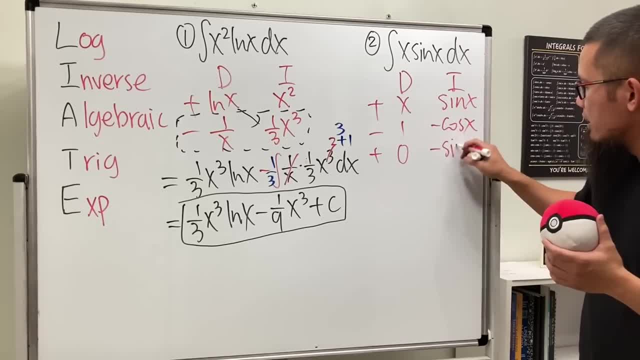 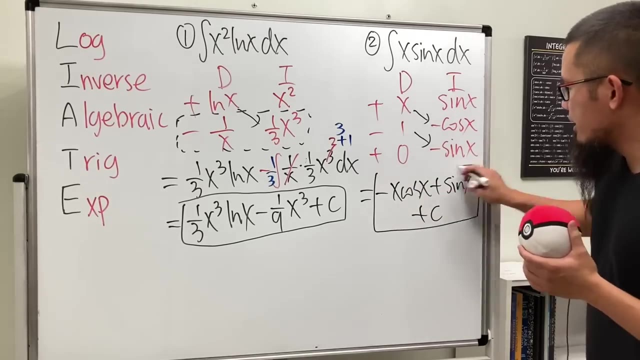 Okay, Do this again, We get zero. Do this: We get negative sine x. Ladies and gentlemen, this times, this, this times, this is the answer right. So we get negative x, cosine x and then plus sine x Done. Then you also put down the plus z right here Again, everybody happy. 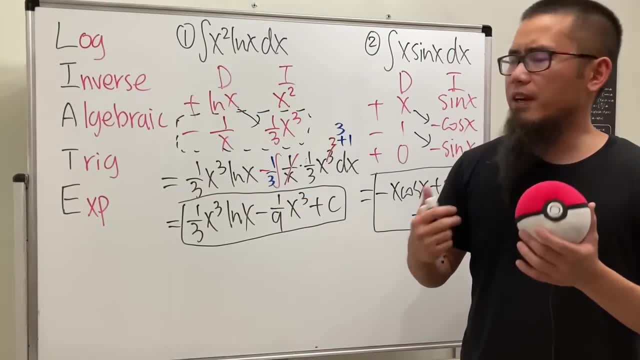 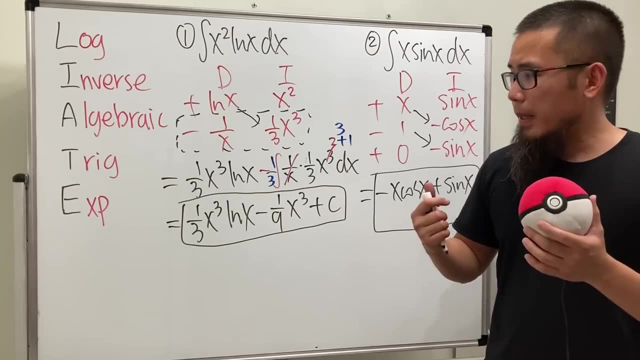 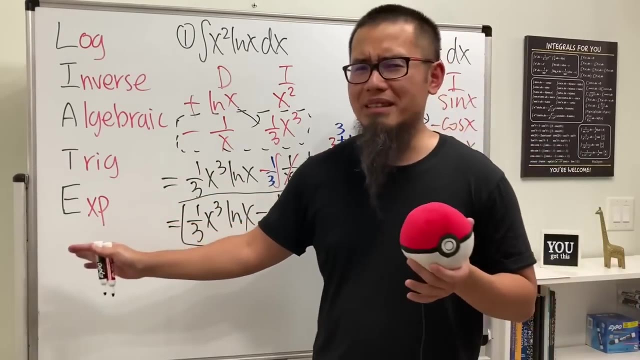 So it seems like this right here is actually very good Tip for us to remember and help us with integration by parts. But first of all I will have to say I agree. This right here helps about like 80% of the time. 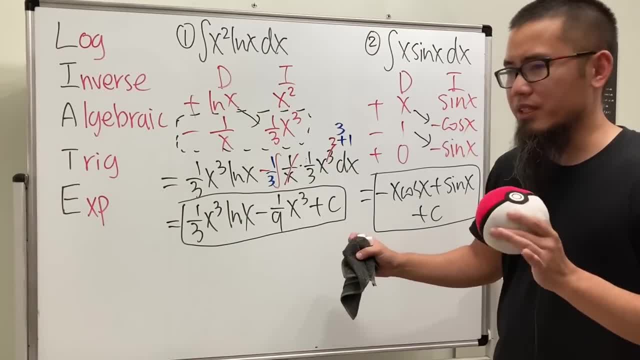 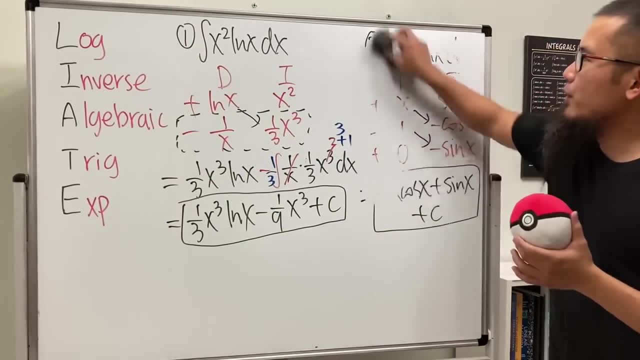 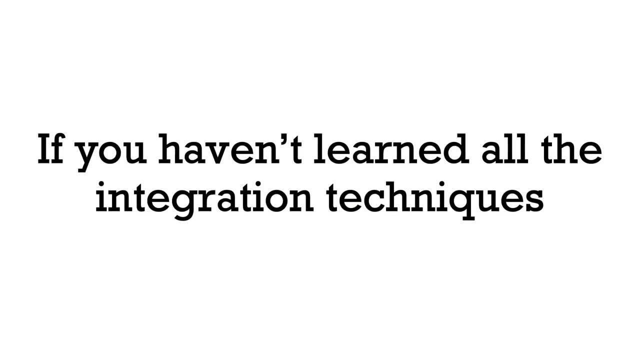 I will say the majority of the classic calculus to typical homework questions. Yes, this right here will definitely be helpful, But if you are trying to do some like a hard to questions, that that Not really Okay. Not really. If you haven't learned all the integration techniques, then you should check out our sponsor today: Brilliant. 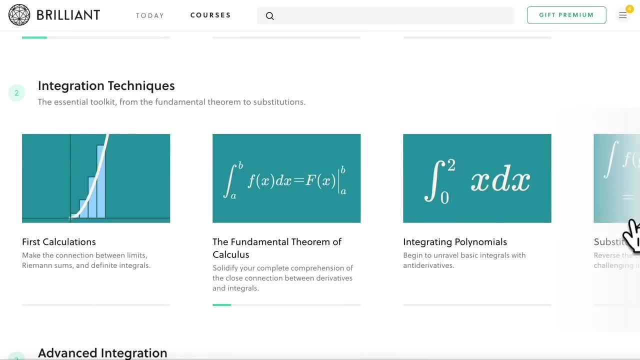 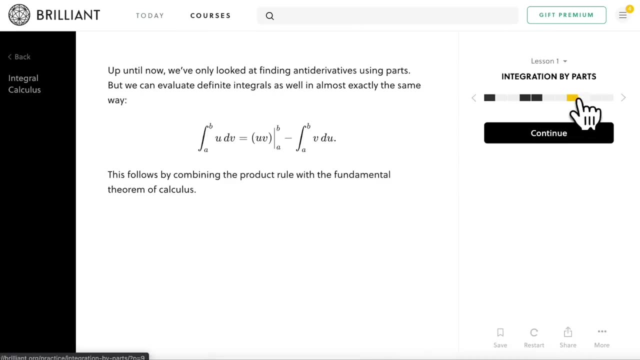 We are currently looking at the integral calculus course. Here they cover all the integration techniques that you have to know, such as integration by parts and different kinds of substitutions. Taking a course from Brilliant is really fun because they will keep you engaged by storytelling and cool animations. 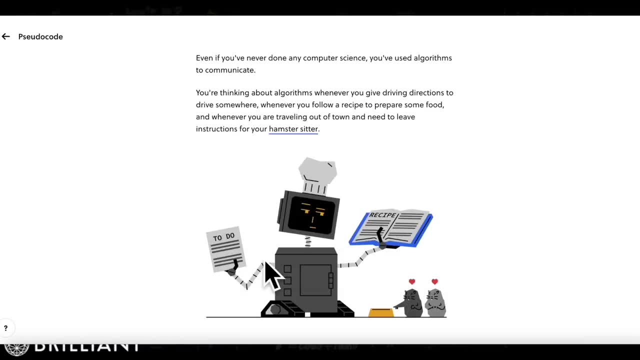 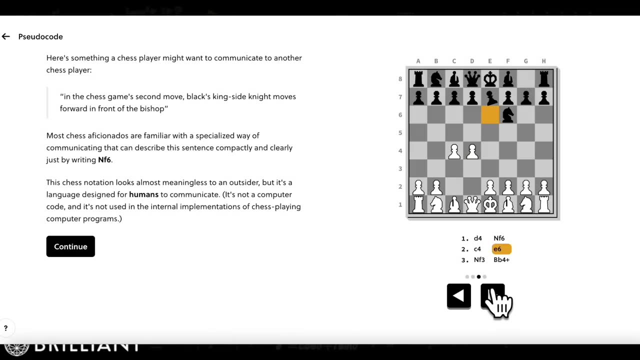 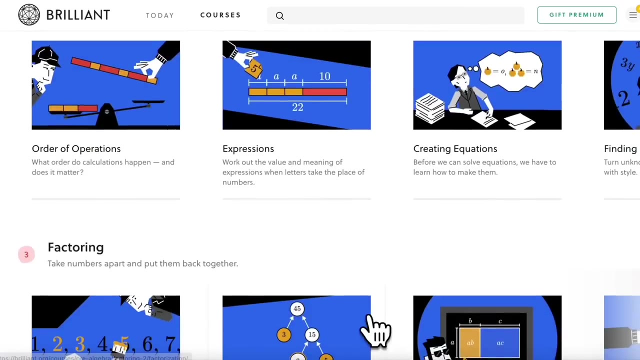 Over the past year they have built a whole new platform for their courses that takes interactivity to the next level. You will see hands-on, You will see their activities while you go through their courses. And especially, they have over 60 interactive courses in math and science and they range from beginning level to advanced level. 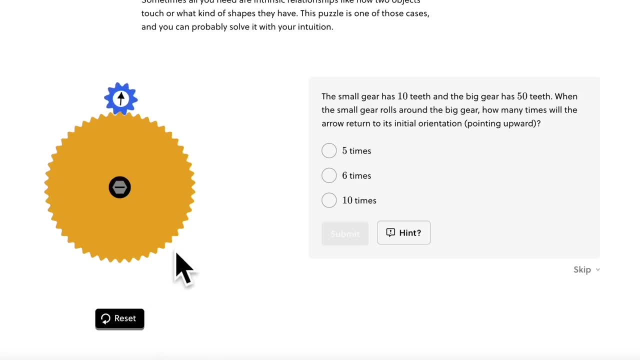 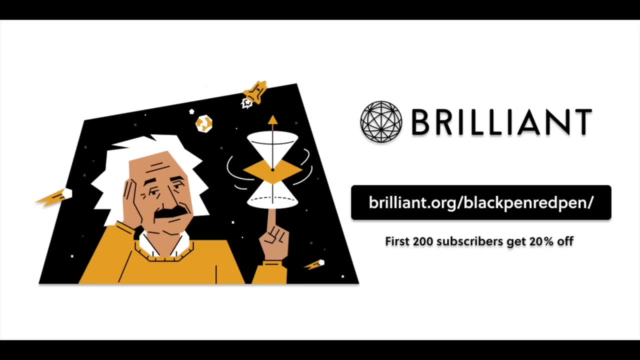 So you will be able to find courses that you like and you can start learning something new and have a special link for you guys: Brilliantorg slash BlackPenRedPen. If you use the link, you will have a 20% off. discount. 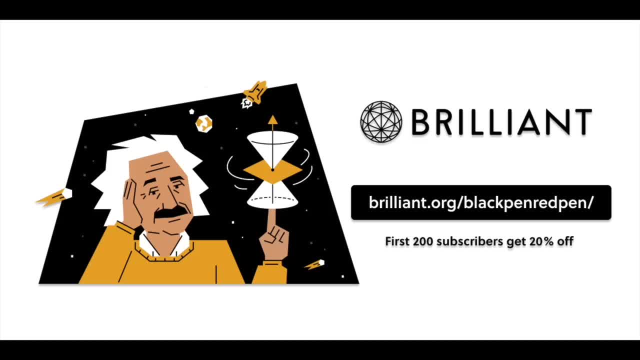 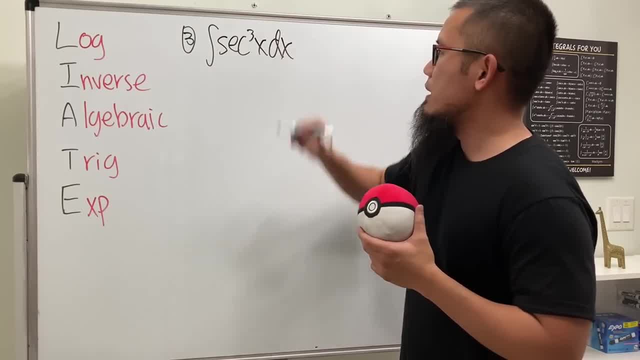 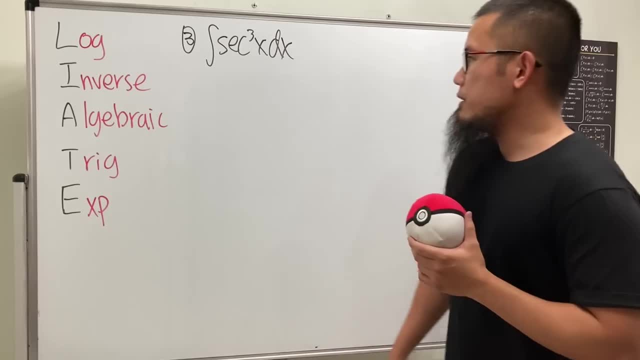 So go ahead and check them out, And I want to thank Brilliant for sponsoring this video. Number three, let's look at the integral of C-CAD to the third power X. We actually have to use integration by parts. First off, we are going to break this apart into C-CAD to the first power times, C-CAD to the second power. 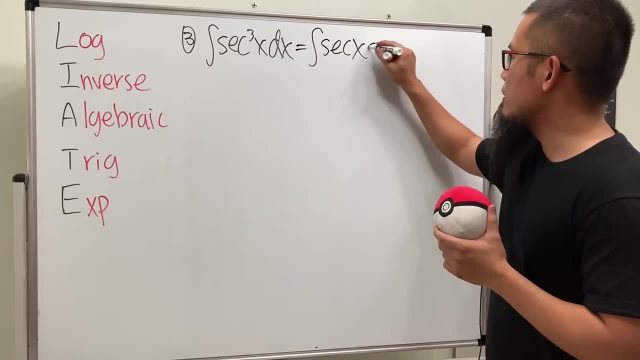 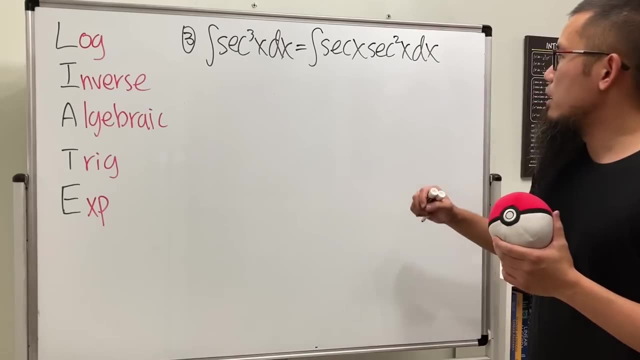 So let's see how it looks like. So let me put this down right here, first, and then C-CAD to the second power. Now we do have two parts And, by the way, do not replace this with a tangent squared plus one. 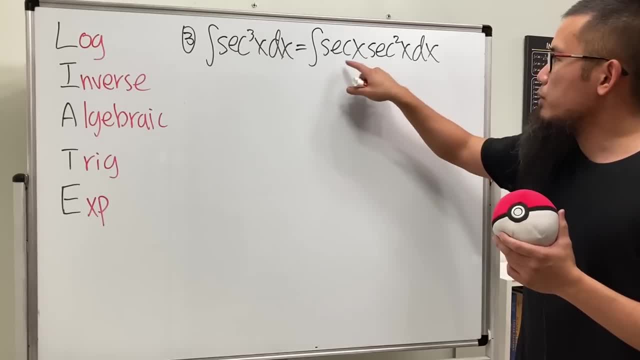 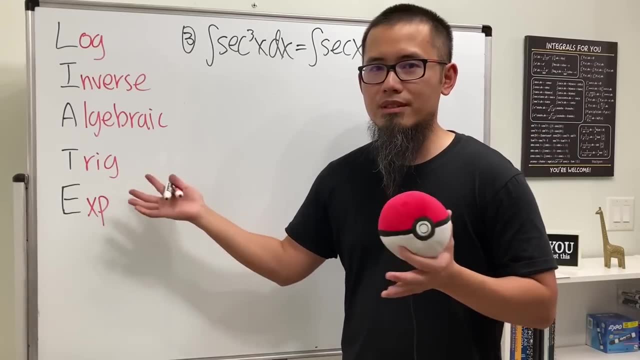 It's not going to help. We have to use integration. But anyway, we have C-CAD to the first and then the other part is C-CAD to the second. They are both trig functions. Which part should we choose to be differentiated? 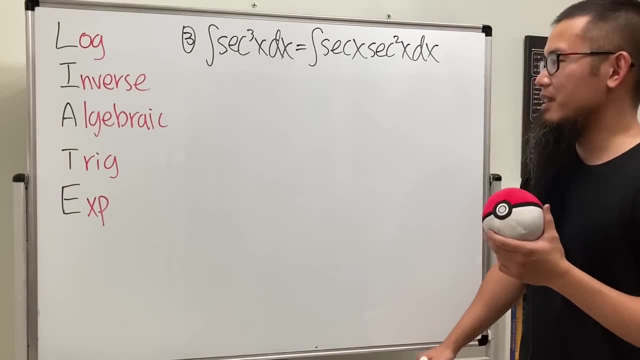 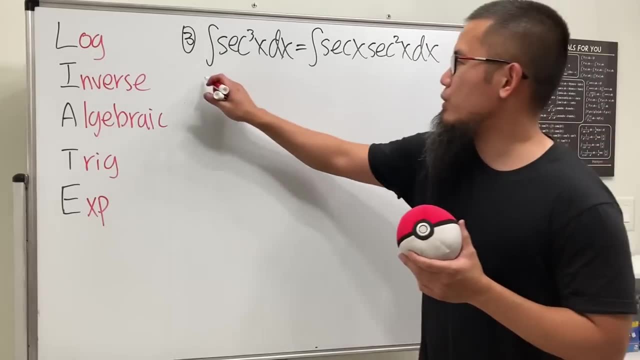 Right. So this is one of the things that huh Yeah, But anyway, here is the video. I really really like to tell my students that when you do the integration by power with the DS setup, like here, always, Always. 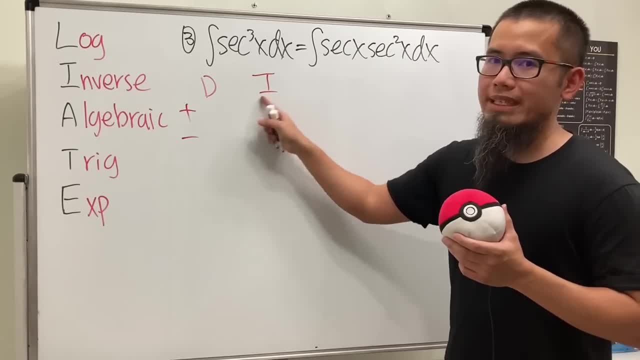 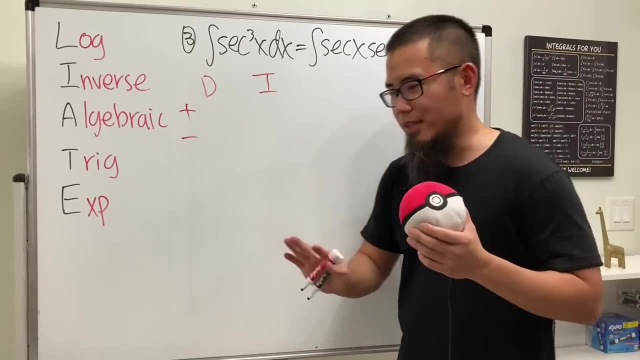 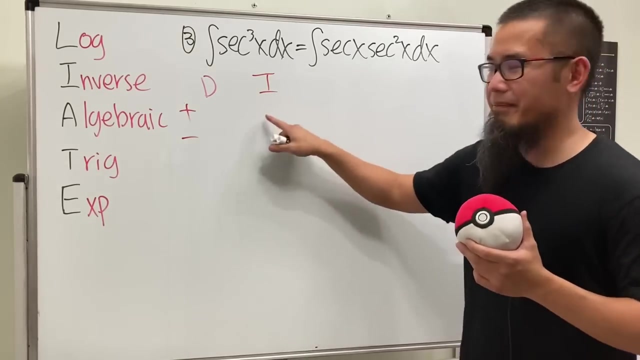 Always, Always, pick the part to be integrated first, because it's always harder to integrate something, right? Well, maybe that's not true. I actually just remembered it's not true. But yeah, anyway, it's usually harder to integrate some of these things rather than differentiate. 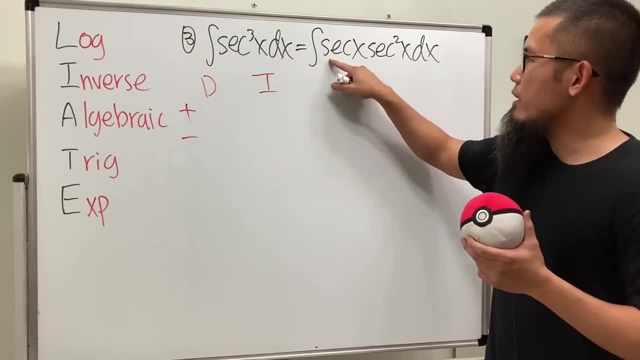 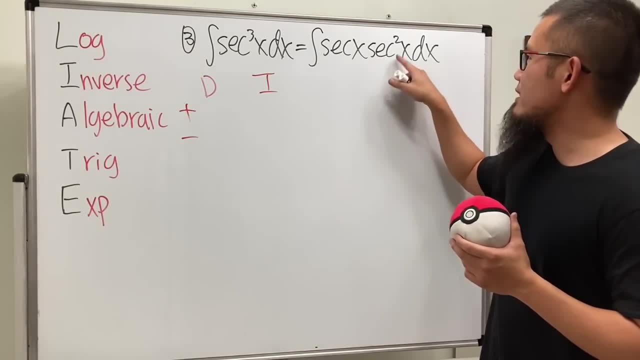 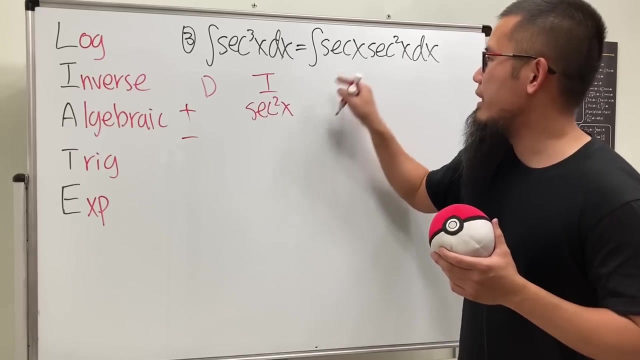 So just ask yourself: can we integrate secant X? Yes, But is it easy? No? Can we integrate secant squared X? Yes, Is it easy? Yes, So we will be integrating secant squared X and let's just differentiate secant X. 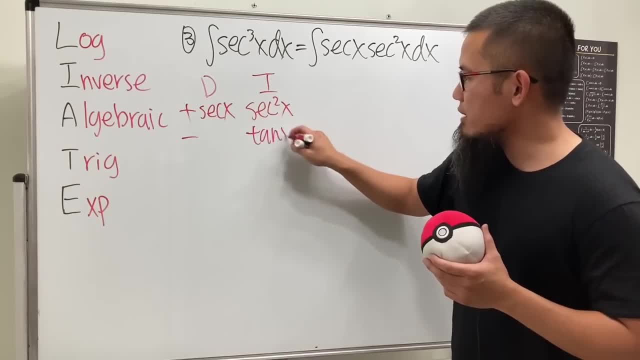 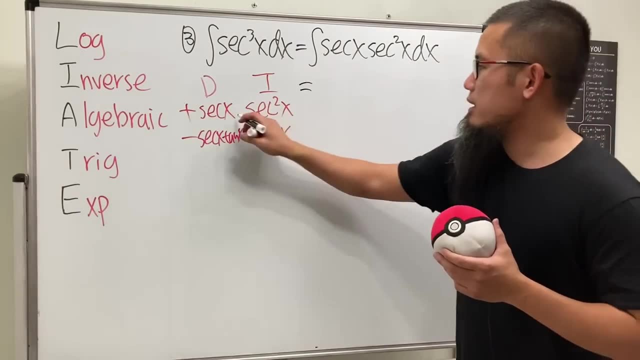 It works. So, integrating this, we get tangent X, and differentiating that, we get secant X, another tangent X, Ladies and gentlemen, this times- this is the first part of the answer- and we get secant X times tangent X. 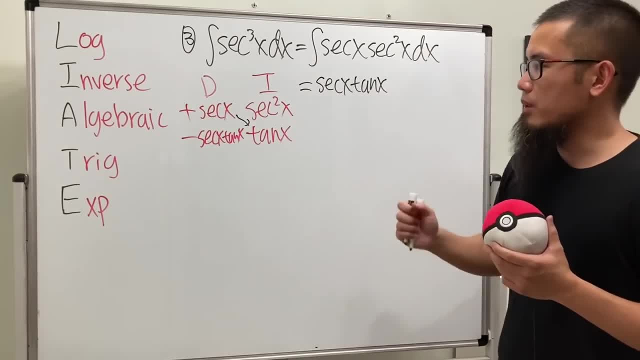 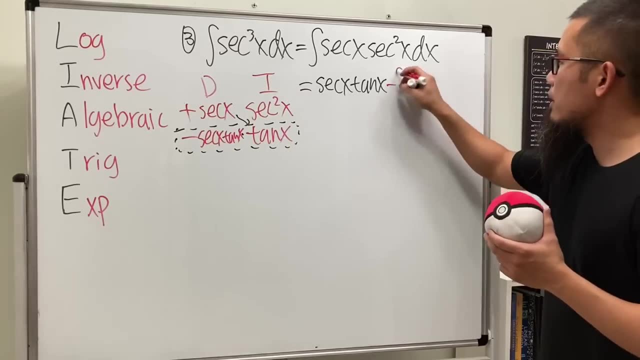 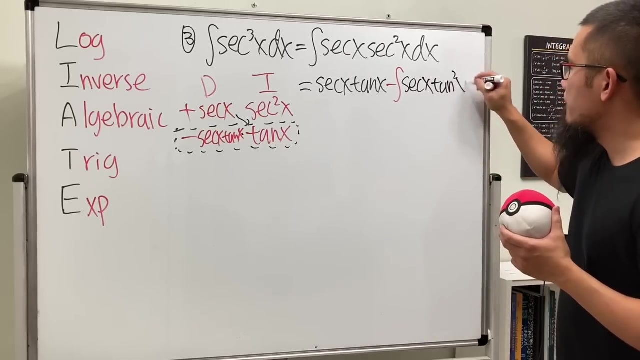 That's how we squeeze out the first part of the answer for this integral. Next, we multiply this. We multiply these two things together and then put that inside of an integral. It's a minus integral and we have secant and tangent to the second power. 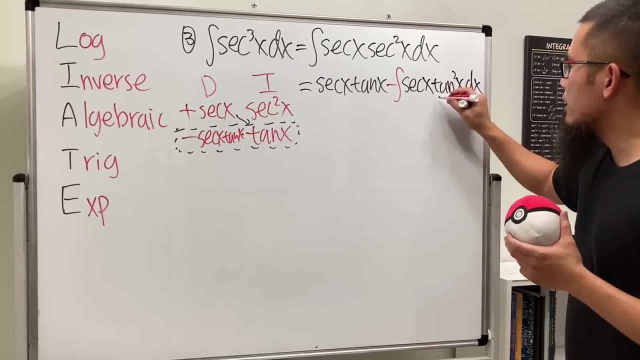 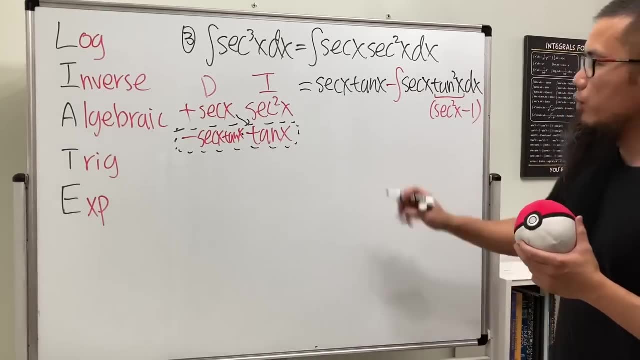 And this is the time that we will be using the identity And tangent squared X is the same as secant squared X minus 1. So if you look at this carefully- I'm going to actually write this down again because you will see- 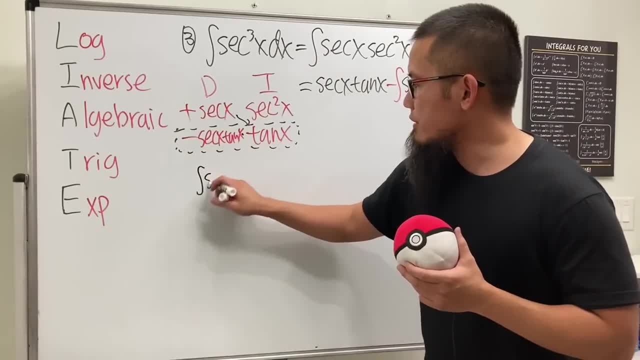 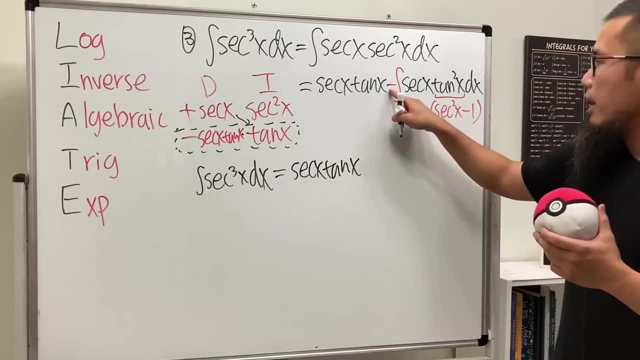 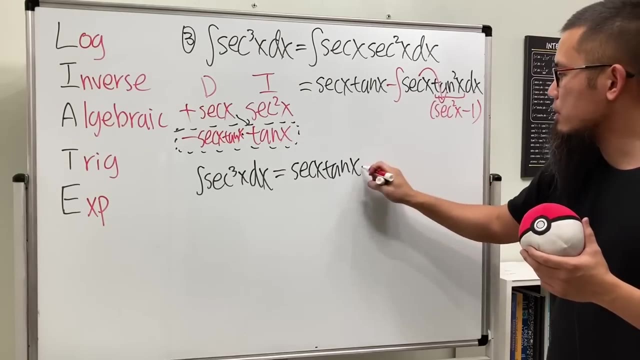 actually a repeating case. so we are looking at the integral of secant to the third power x, dx. that's equal to that. secant x, tangent x. this right here is inside of the integral, but we will have to distribute the secant to here so we get minus integral of secant to the third power x. 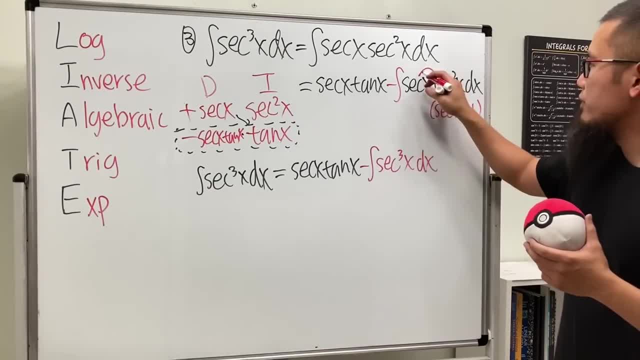 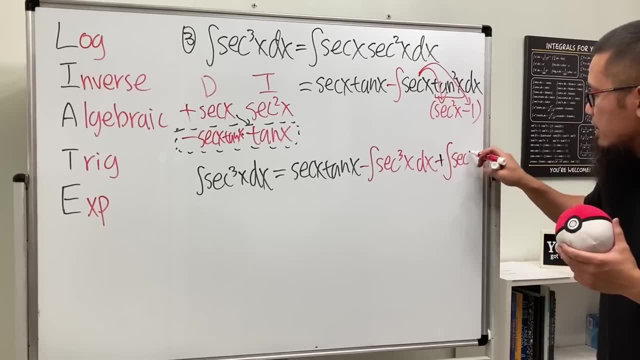 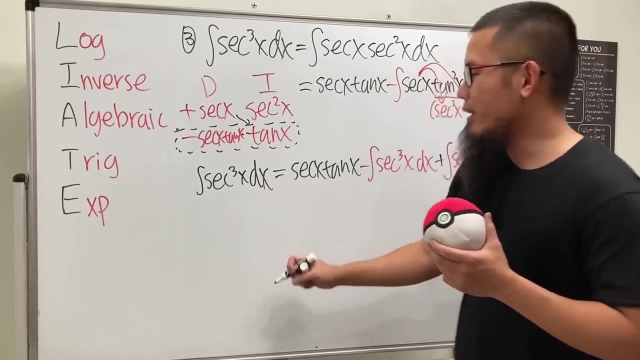 and then dx that and we will also have to distribute this to that and negative, negative so becomes the positive here integral, and then we just have secant x dx. now you see this. we can just move that to the other side and we'll end up with two integral of secant to the third power x. 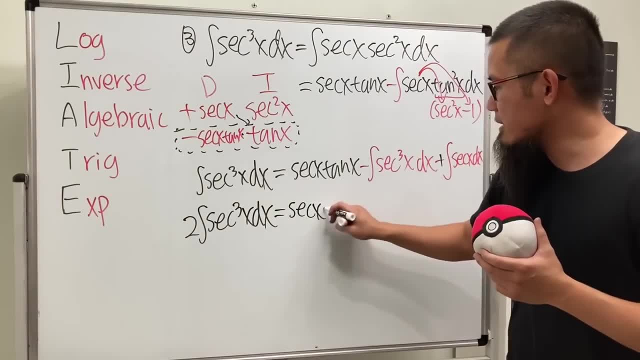 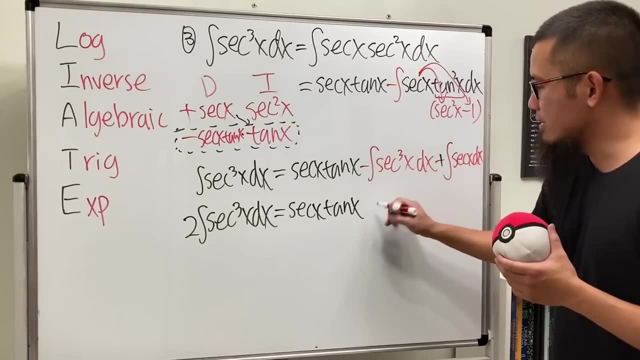 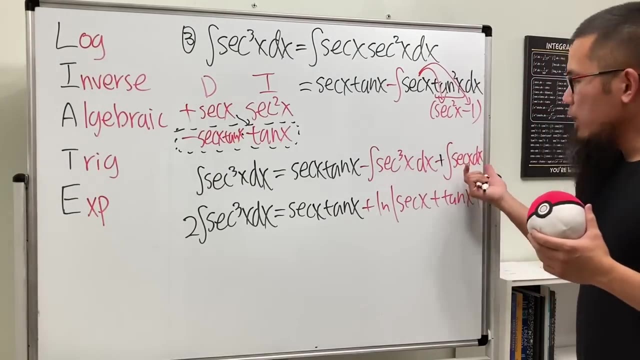 dx and you see, this right here is just secant x times tangent x, and this is over there already and this right here it's a standard result and we just know that that's going to be ln abs, the value of secant x plus you tangent x. if you really want to put secant x right here, yes, you can integrate that just by. 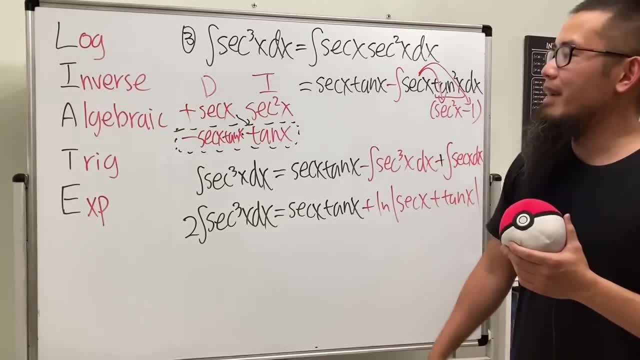 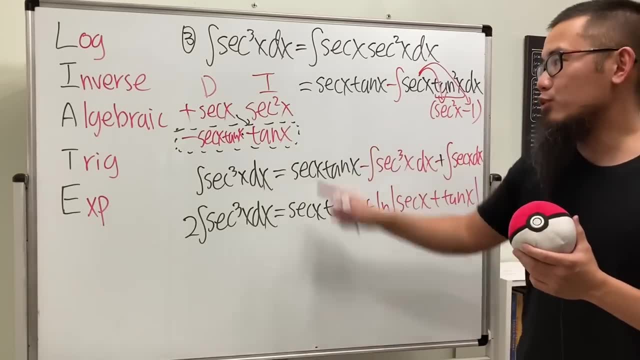 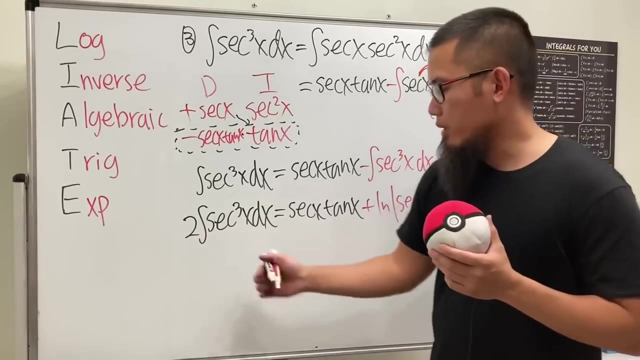 putting down a standard result. but once you multiply the second row, the two things from the second row, yeah, no, that's why, right, always think about what to choose to be integrated first. but anyway, we are not done yet, because we don't want this two right here. so divide everybody by. 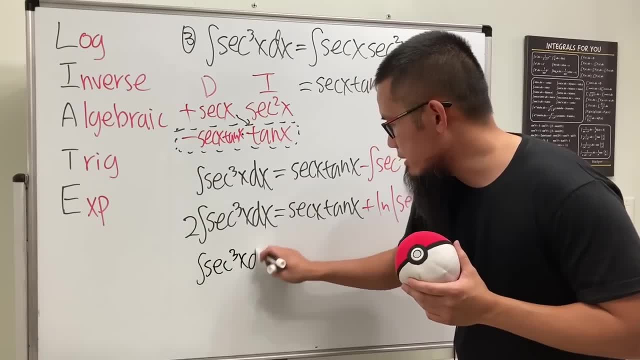 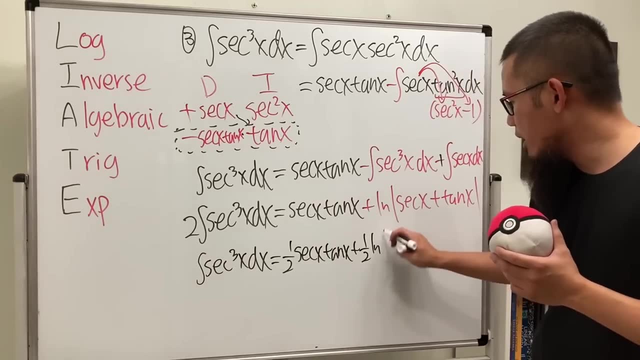 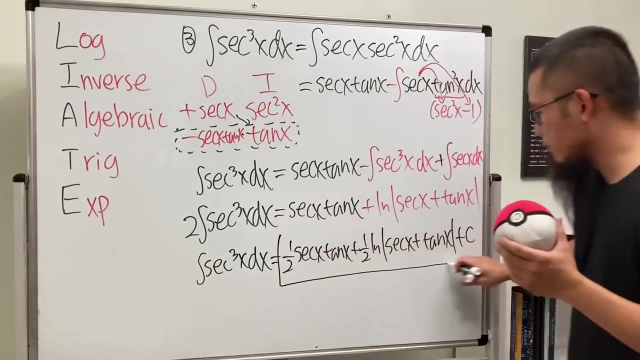 two. therefore, the integral of secant to the third power x dx is going to be minus. integral of secant to the third power x dx is equal to one half secant x, tangent x plus one half ln abs, the value of secant x plus tangent x, and then of course, plus c, we are done. 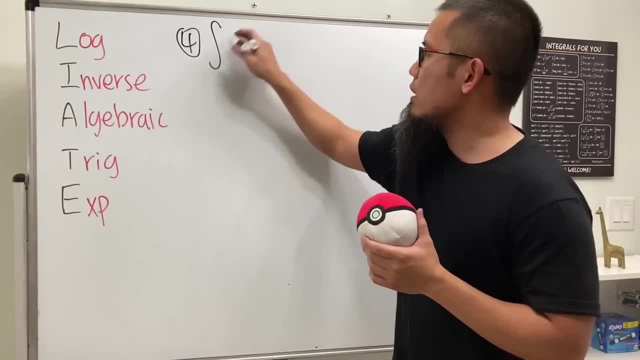 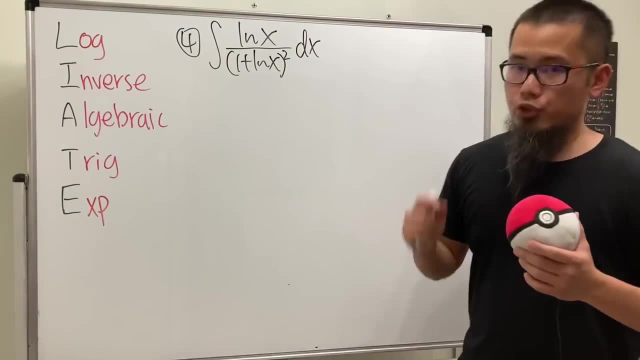 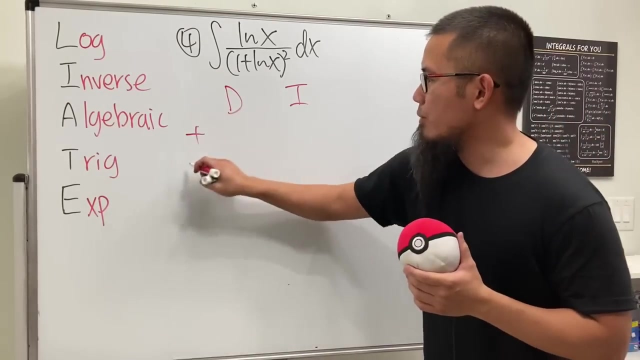 okay, this is number four. let's take a look at the integral of ln x over 1 plus ln x and then square dx. trust me, we do integration reports with this one, all right. so let's go ahead and put on d and also the i plus or minus, and thanks to this, okay, we. 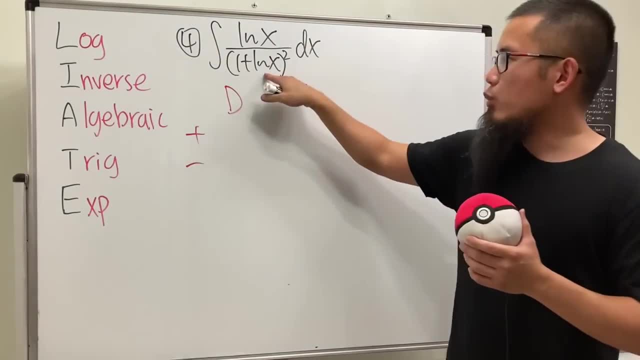 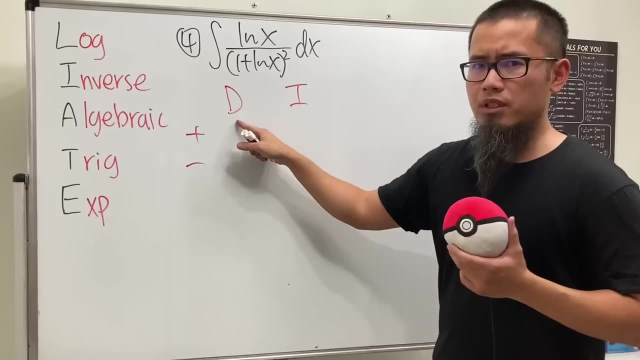 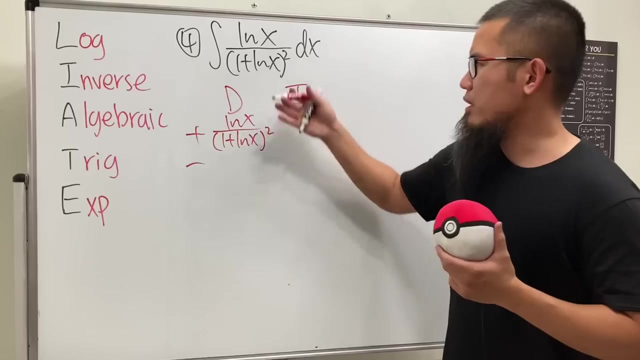 see ln x, which is the natural log function, and likewise we also have the natural log on the bottom. so it seems like we should just put the whole thing down to be differentiated: ln x over 1 plus ln x and square, because both of them have the log right, wow. 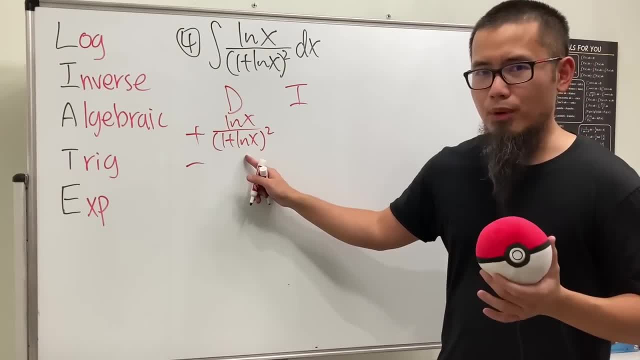 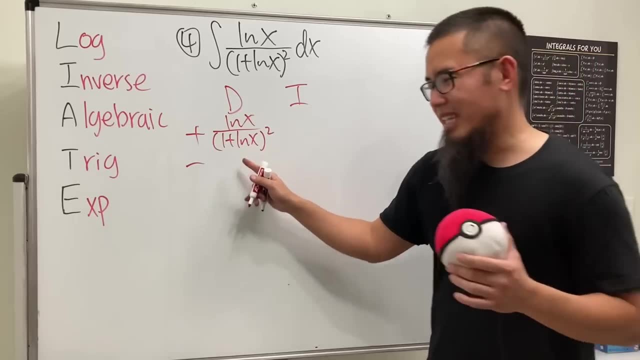 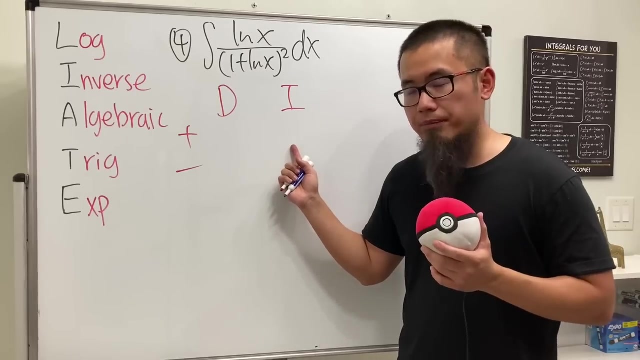 do you really want to differentiate this? it's doable, but do we really have to? is life that hard? you guys can let me know? we really just have to think about which part we should choose to be integrated first, and we have to do it carefully. should we just put down ln x right here to be integrated? no, because we have to do. 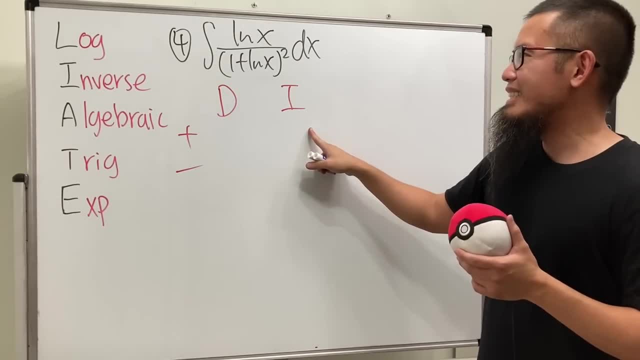 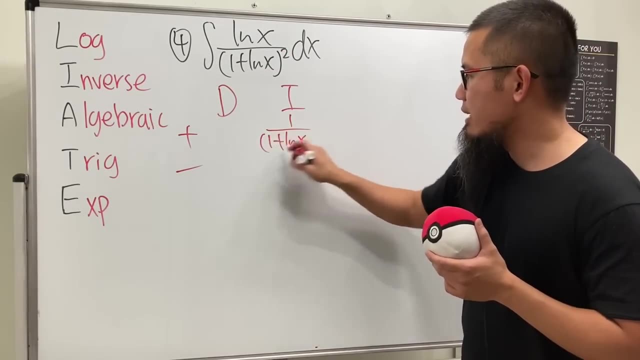 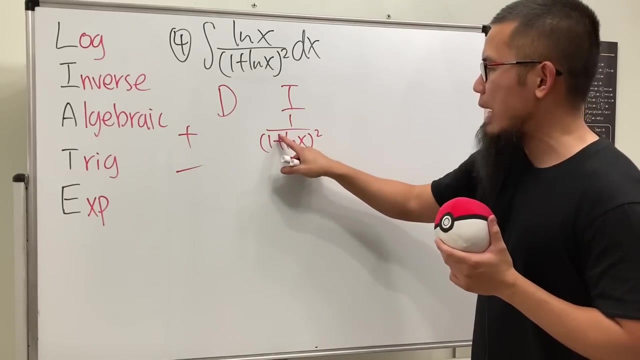 integral parts for that right technically. uh. so the stemming we should just put on the rest. and this is on the bottom. so let me write down: 1 over 1 plus ln, x and a square. can we integrate this? no, but what if we try to do you sub, let u equal the inside. 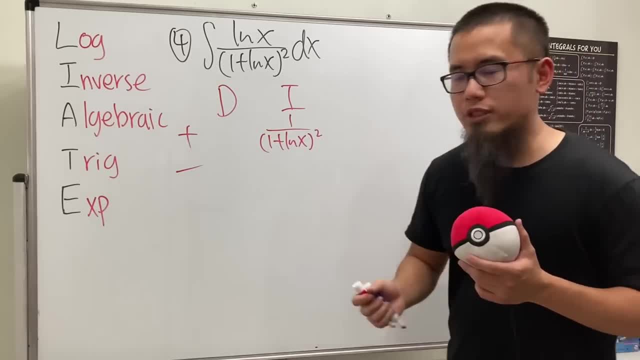 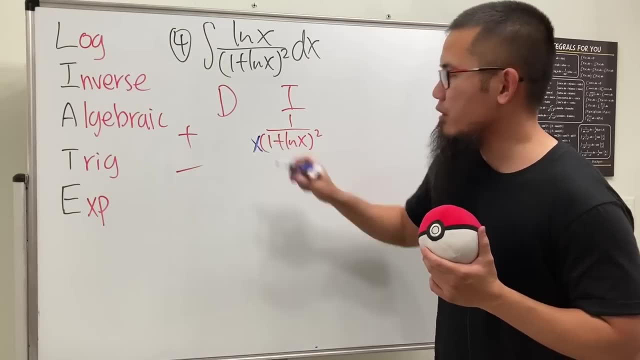 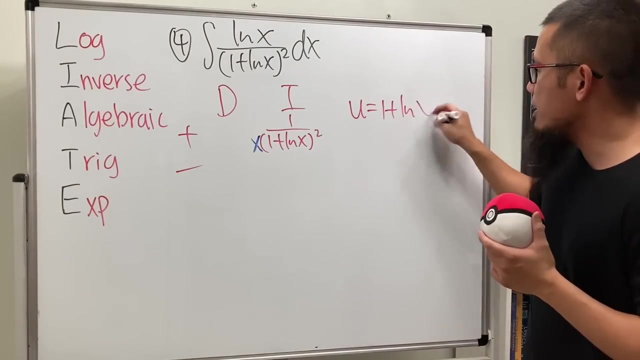 where the derivative of the inside is one over x. Unfortunately, there's no x, But now just think about it. Wouldn't it be nice if we happen to have an x right here? Yes, it would be so nice, Because then we can just proceed by u sub du equal 1 plus ln x. 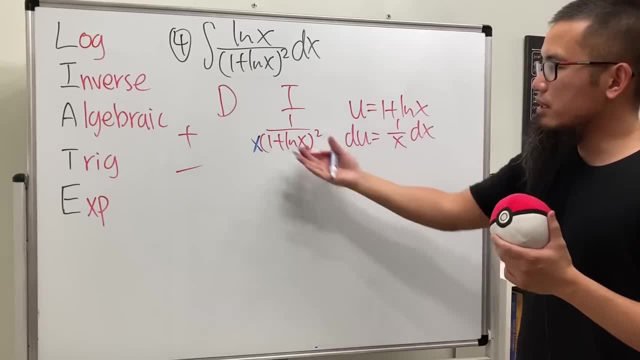 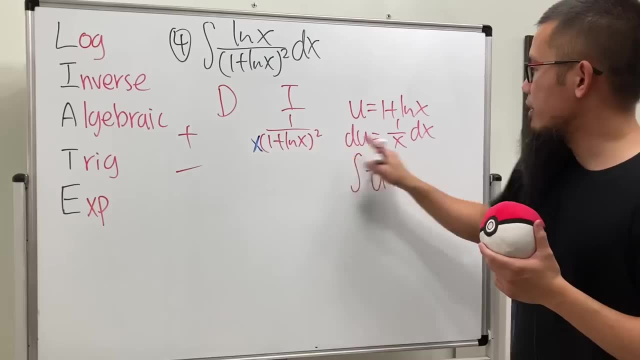 And du is just equal to 1 over x, dx And you see, this integral becomes the integral, And then we have 1 over u squared And this right here, and the dx. imagine that This is just going to be the du. 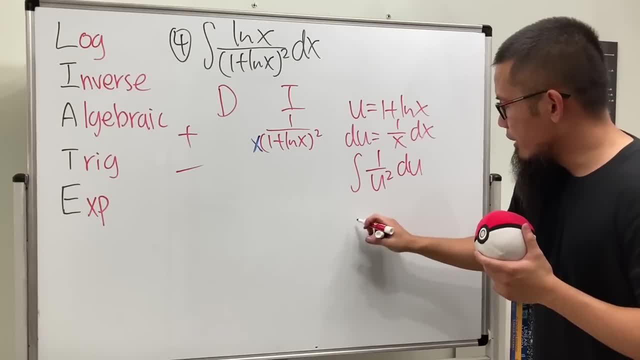 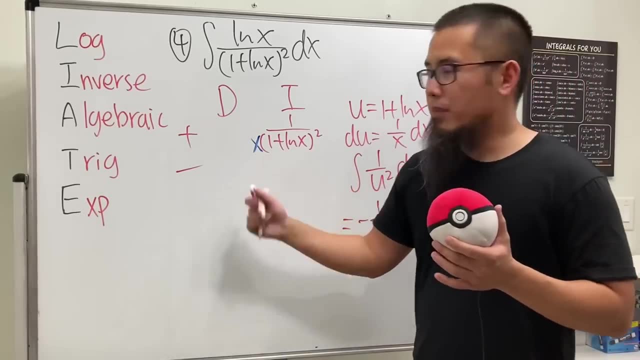 And this right here is just going to give us, you know, negative 1 over u to the first power, right After you integrate that. So this right here now is doable, But we didn't have the x in the beginning. 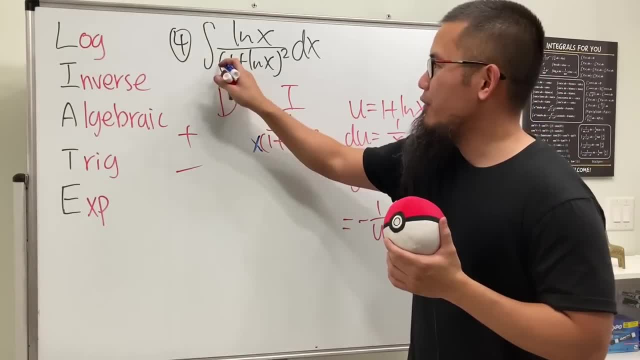 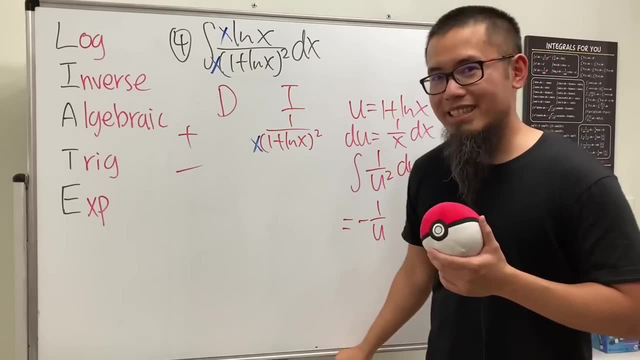 Don't worry, Let's just go ahead and do the following: If you don't have it, multiply by that And don't forget to do the same thing on the top. So now, if we actually just do that, you see, we have the bottom portion right here. 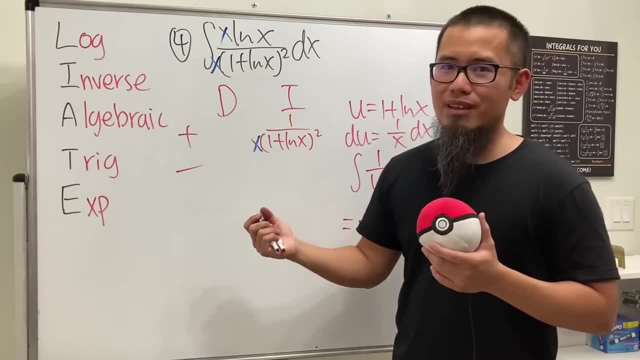 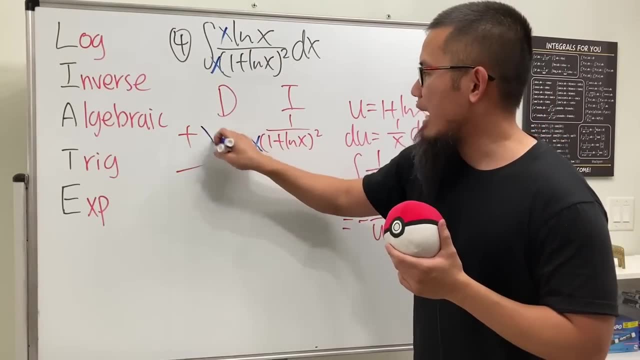 That That part is to be integrated. So what does that mean? That means we should just take the top part to be differentiated. So let's go ahead and do that. Here we have the x times, ln, x. Yes, very nice. 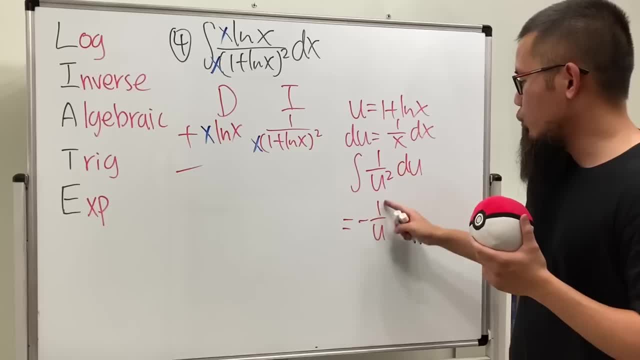 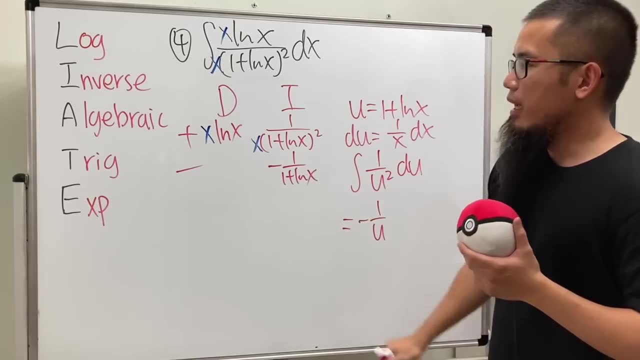 Check this out. When we integrate this guy, it's just negative 1 over u And u. is that? So we end up with negative 1 over 1 plus ln x, And when we differentiate this guy, we use the product rule. 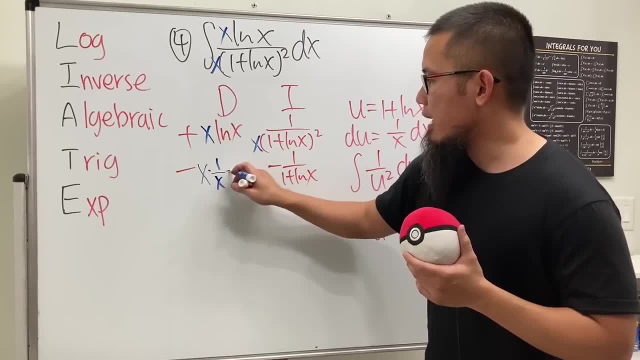 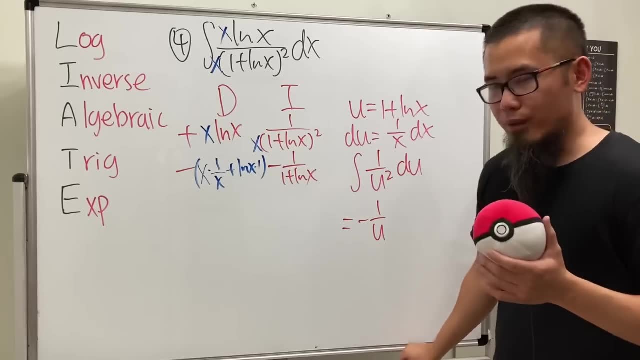 So we do x times the derivative of the second, plus the second function times the derivative of the first, which is just 1.. Just like that, right? And now let's construct our answer like the good old way, right? So we do: this times this: 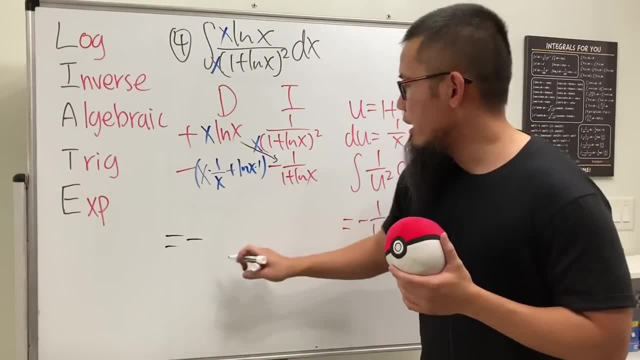 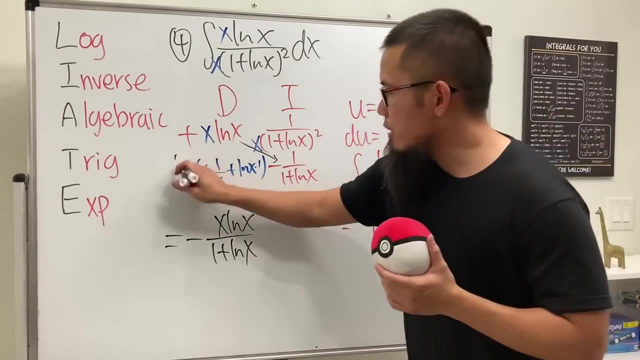 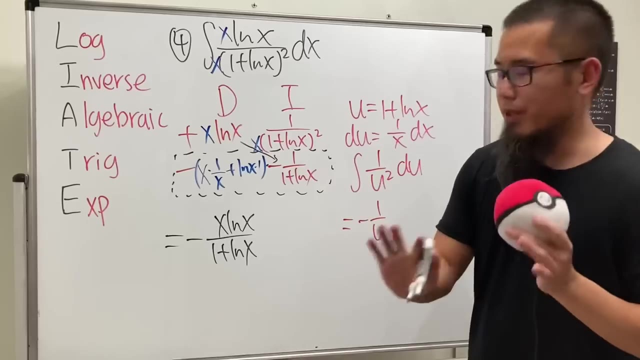 That will keep us the first part of the answer. So we have negative and we have x ln, x over that on the bottom And we are going to be multiplying these two things together. But check this out: Negative times negative is positive. I know, I know, I know. 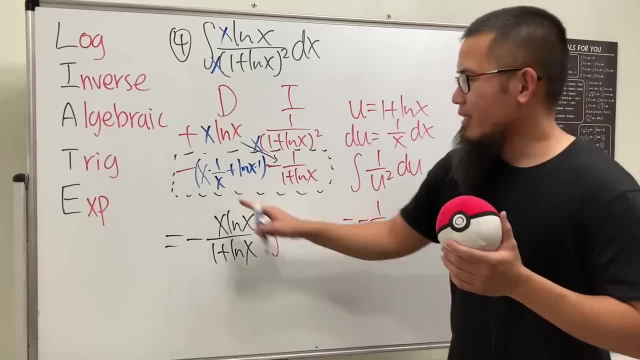 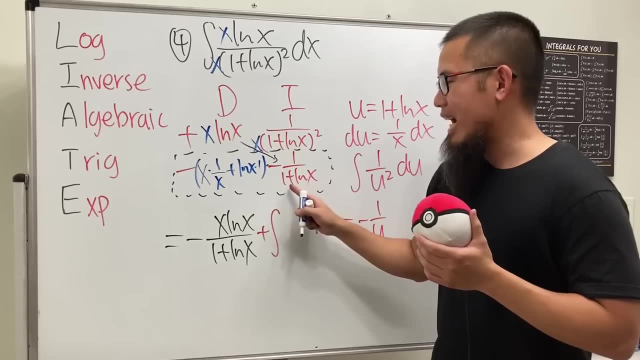 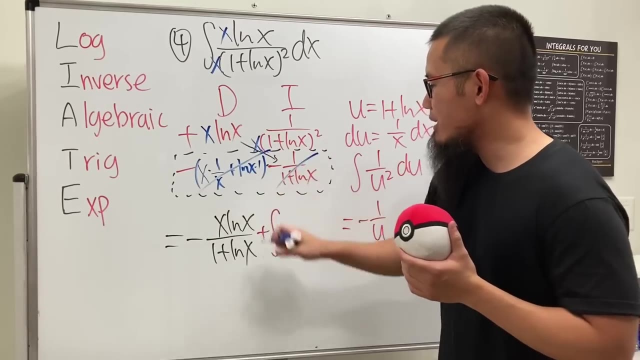 But let me just say that Plus the integral. Check this out. What's this? This is just 1, and then plus ln x. Here we have 1 plus ln x. When you multiply this, they cancel each other out. So in fact we just have a 1 right here and we have to differentiate that right. 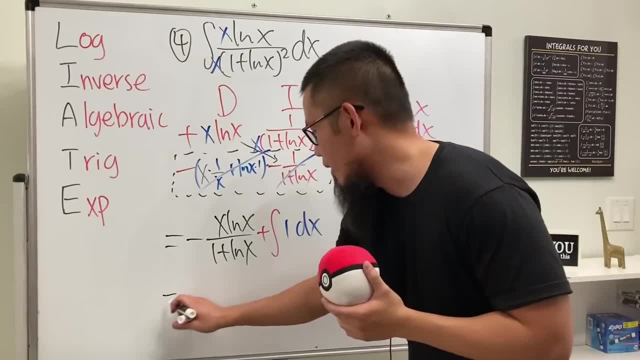 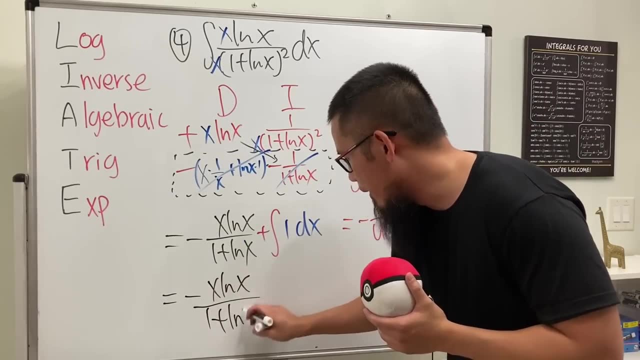 So this is so wonderful Because this right here It's just going to be plus 1 in the integral. So this right here is negative x, ln x over 1 plus ln x, And then we just need to add the x, We are done. 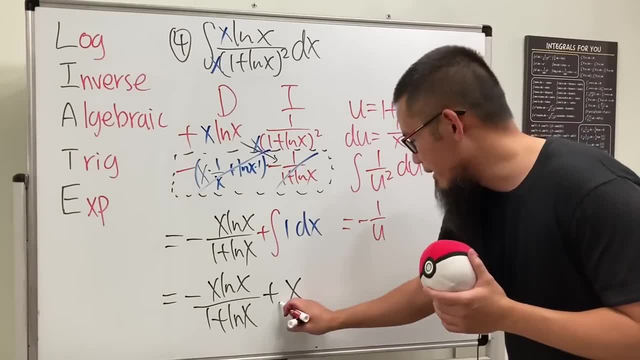 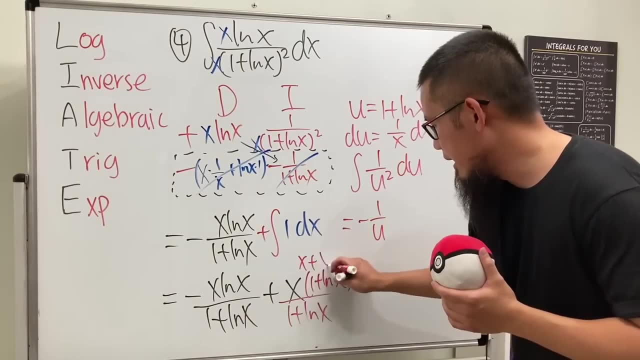 But I can make it slightly prettier for you guys, because this right here actually simplifies really well. Let's multiply the top and bottom by 1 plus ln x And then you see, this right here is just x plus x ln x. When we combine this and that, cancel. 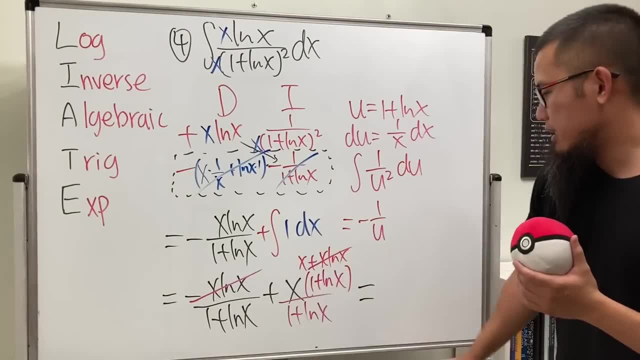 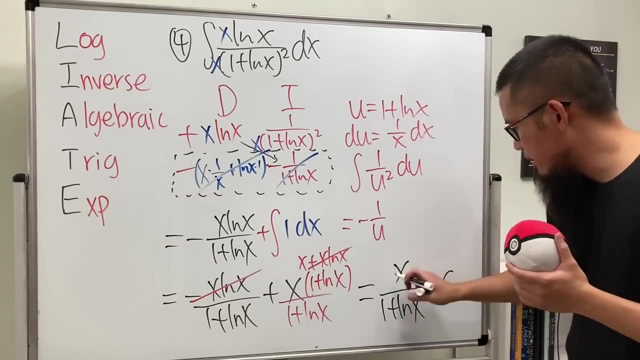 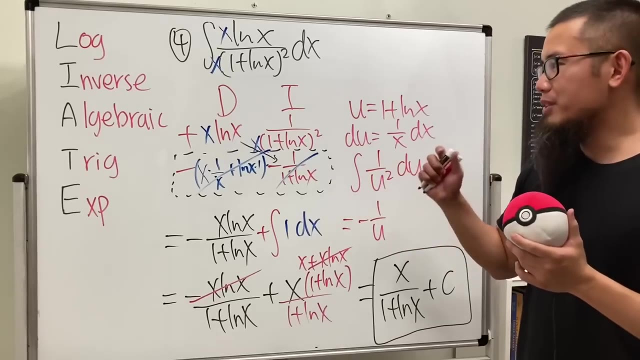 So, ladies and gentlemen, This right here actually gives us x on the top over that, x over 1 plus ln, x plus c. We are done. So, yeah, This is what I like to show my students. They just have to really think hard on which part that they should be choosing from the.